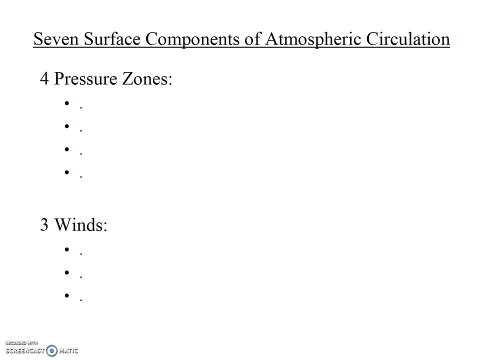 The model that we're going to develop in this video clip still does have three winds and very much the same way that the previous model did, But we're also identifying four pressure zones. I encourage you to pause the video for a moment and write down these four pressure zones and these three wind systems. 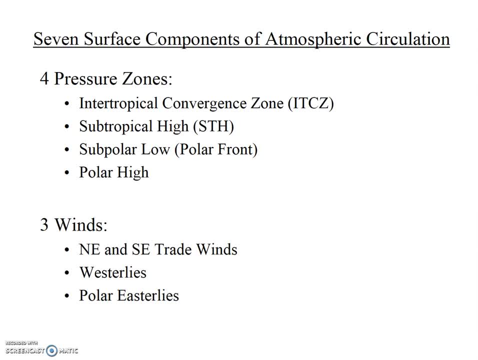 tropical convergence zone occurs near the equator. Subtropical highs are located at or near 30 degrees north and south. The subpolar low, which your book calls the polar front, is located near 60 degrees north and south, and the polar 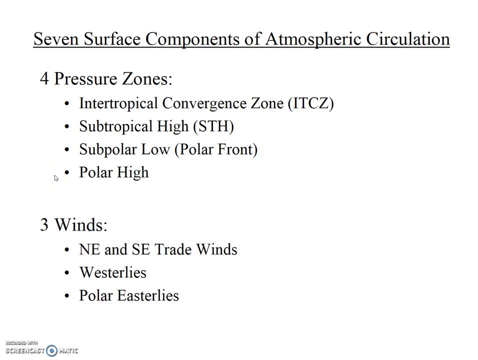 high is located near the poles, at 90 degrees north and south. The three winds are always flowing, from high pressure to low pressure. The trade winds flow from the subtropical high to the intertropical convergence zone at the equator. The westerlies also flow from the subtropical high, but they flow 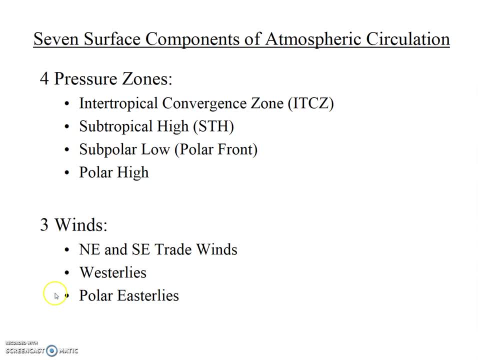 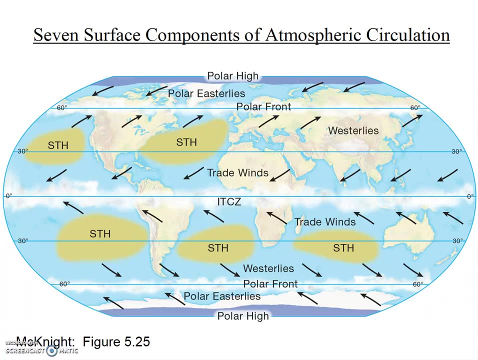 towards the polar front, And the polar easterlies flow from the high pressure at the poles to the polar front. Now that you've written the seven components down in your notes, take a look at your notes and identify all seven components on this diagram. 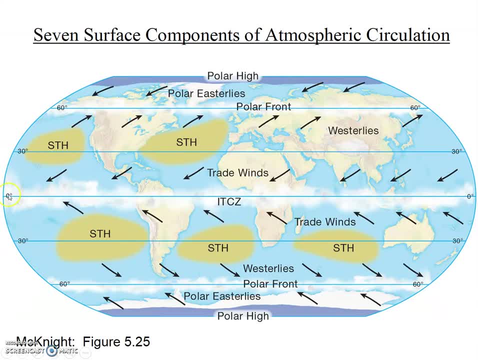 Start with the pressure zones, the intertropical convergence zone here at the equator, subtropical highs, the polar front and the polar high. Then notice the winds, the trade winds blowing towards the equator from the subtropical highs, the westerlies blowing from the subtropical highs towards the. 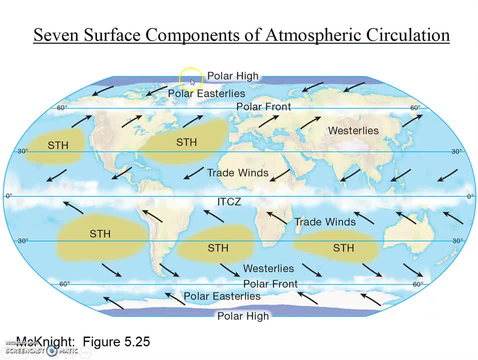 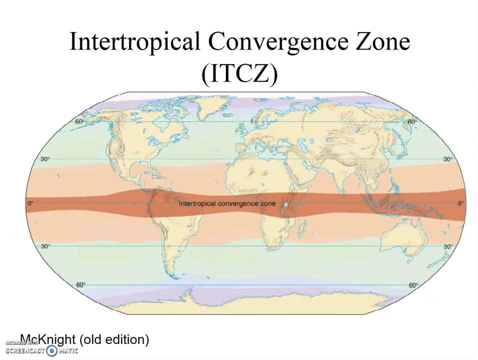 polar front and the polar easterlies, from the polar high to the polar front. Again, winds are always blowing from high to low pressure. We're gonna go through each of these components now in more detail, starting with the intertropical convergence zone, The name: 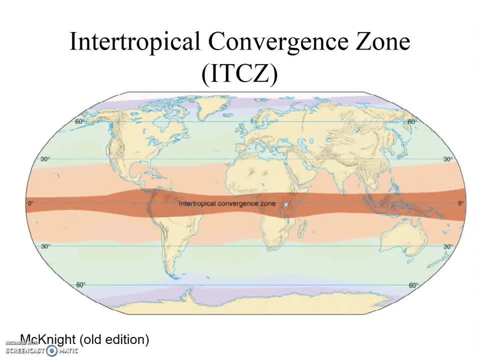 of the intertropical convergence zone is very descriptive. It occurs near the equator, That's, within the tropics, inter-tropical, and it's a region of converging air. remember from our last video clip that airflow around a low-pressure cell in the Northern 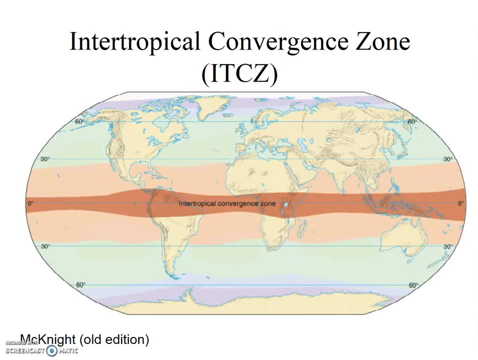 Hemisphere is counterclockwise and convergent, So air is flowing towards the equator. As we have previously noted, warm equatorial air expands and rises, thus creating a low-pressure zone. So the intertropical convergence zone is a low-pressure zone. Within the ITCZ, the weather is warm, calm and cloudy. The 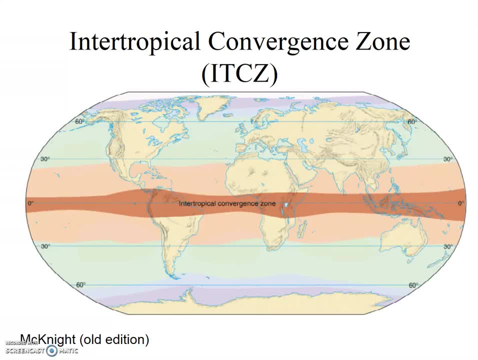 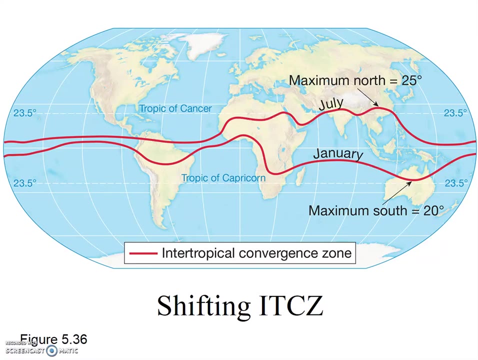 dominant air movement is upward, not horizontal, and the rising moist air cools to form clouds. Notably, the ITCZ moves north and south a bit with the seasons. It's not always exactly over the equator. The movement is more. 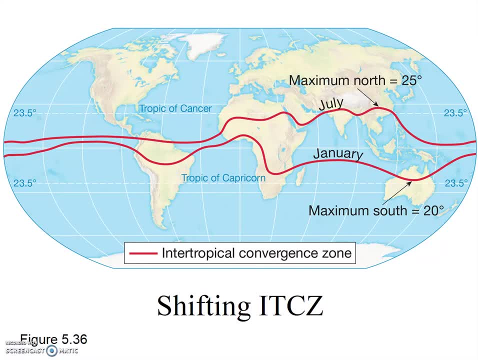 probable than we think. Thisalımatically stays仰 JP Canada Because it is the third Os. Tales of Hurricane� isn't always exactly over the Equator. The movement is more pronounced over the continents than over the oceans, because the continents tend to heat. 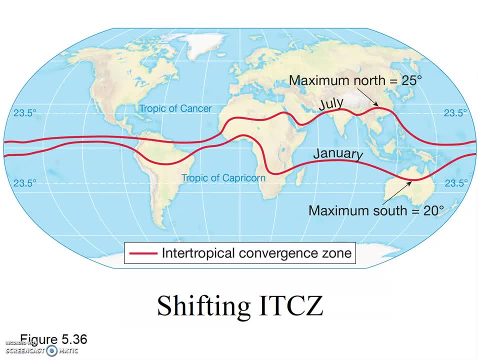 up faster and to a greater extent than the oceans, And warm rising air creates the low pressure cell that makes up the intertropical convergence zone. So the ITCZ is a low pressure zone near the equator with rising air. You can see the ITCZ in this satellite image near 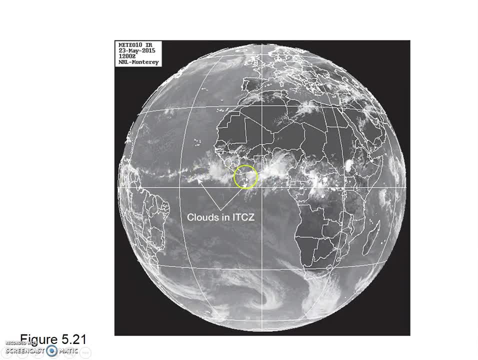 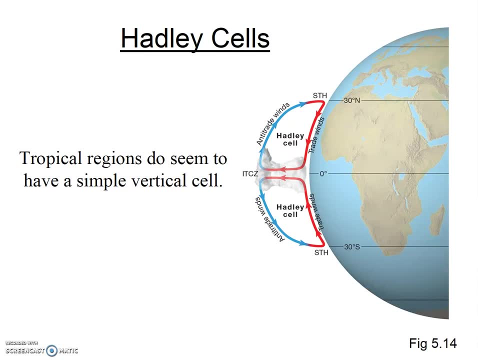 the equator. here, where there is a preponderance of clouds, We noted that the global system does not just simply have a convection cell from the poles to the equator, but indeed the tropical regions do seem to have a simple vertical convection cell. Air rises at the equator at high. 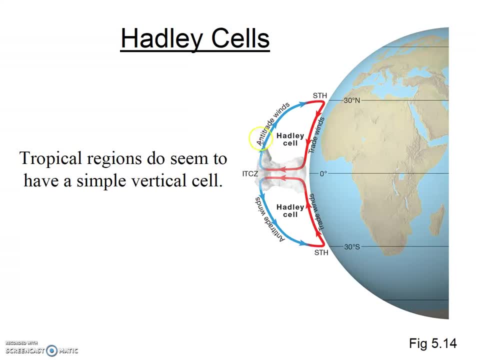 high altitudes The air actually starts to move poleward and it gets colder and it descends at about 30 degrees north And 30 degrees south latitude at what we call the subtropical highs. 30 degrees north and south are high pressure zones because the air is descending upon them. The name subtropical 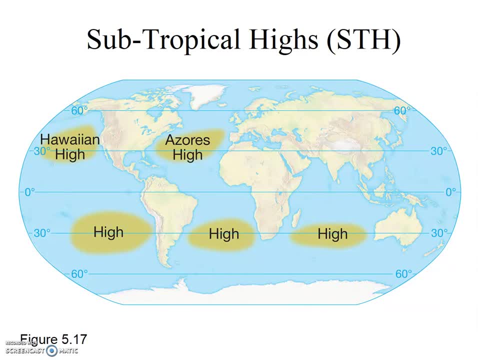 high is quite descriptive. It's a high pressure in the subtropics. that means just outside the tropics, and weather in the subtropical high is calm and clear. The dominant air movement is down, not horizontal. Additionally, in general rising air is needed for cloud formation, Since the air in the subtropical 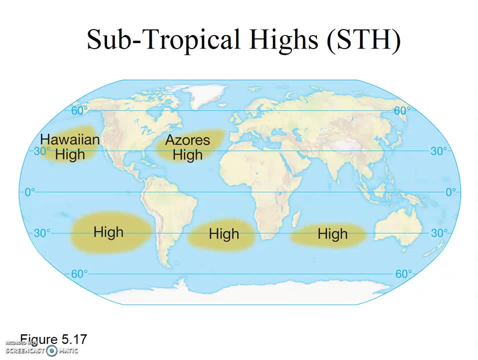 high is descending, there's no clouds and thus no rain. As we noted previously, many or most of the world's deserts are in or near the subtropical high. The subtropical high cells are huge and take up most of the major ocean basins at 30 degrees north and south. Additionally, these cells are: 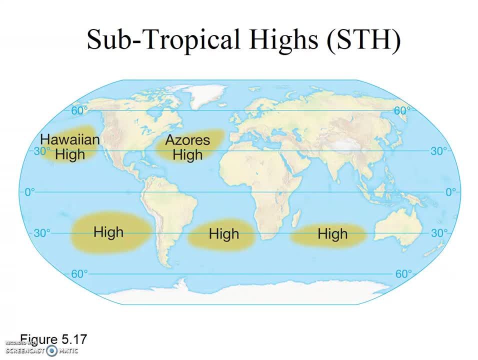 very consistent over the ocean basins, but less consistent over land. Why is that? Well, consider what happens to land within the continent interior. in the summer It heats up and expands and rises. Rising air creates a low pressure cell. Thus in the winter there may be evidence of subtropical 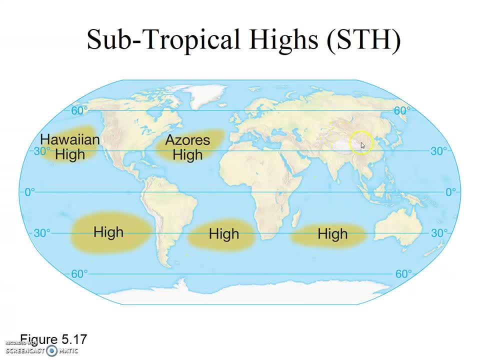 high over southern Asia here, but it's absent in the summer because it breaks up because of the rising air. Also, just as the ITCZ shifts with the seasons, so does the subtropical high. It moves slightly north in northern hemisphere summer and slightly to the south in northern hemisphere. 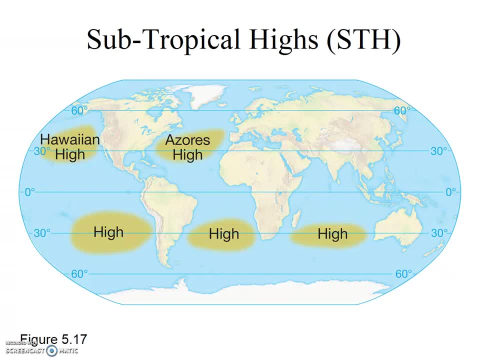 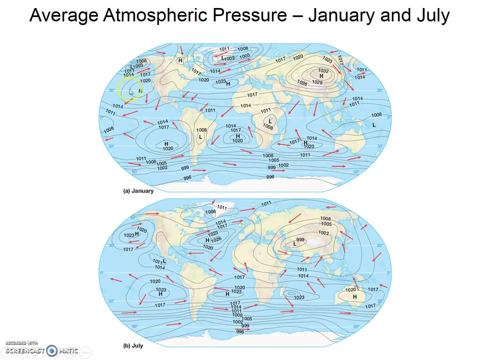 winter, And we'll see that this shift is what's responsible for giving California our long, dry summers. We've now discussed a high pressure zone- the subtropical high- and a low pressure zone- the intertropical convergence zone. Next, let's check out the winds that connect them. 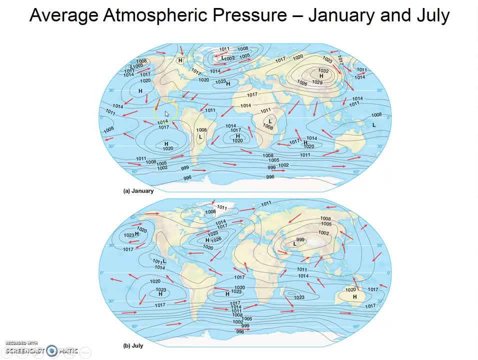 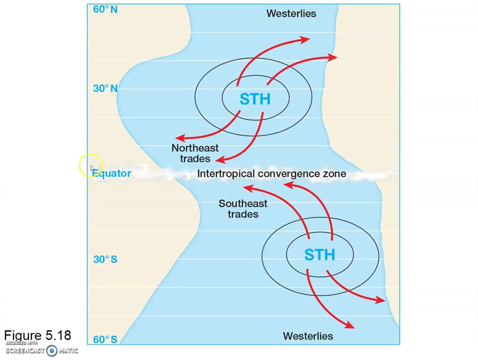 Again, winds flow from high to low. Figure 5.18 in your text is a pretty informative figure. It shows the intertropical convergence zone with its cloudy, rising air, the low pressure, and it shows the subtropical high, around 30 degrees north and 30 degrees south. And then you 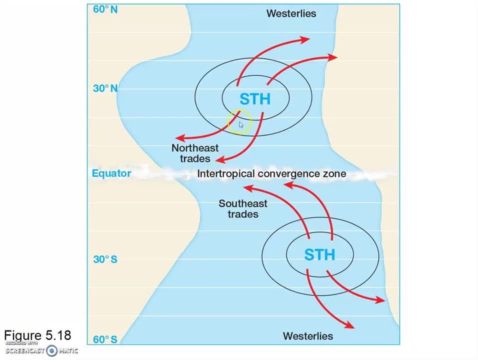 can see that the trade winds flow from the subtropical highs to the intertropical convergence zone. You could say that the northeast and southeast trades converge at the intertropical convergence zone. Notice how these winds are named. We named winds from the direction, from. 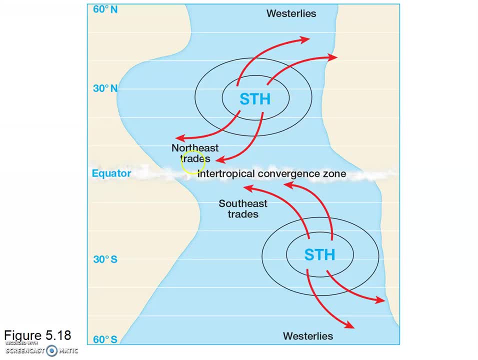 when they come from. So we have the northeast trades and we have the southeast trades. The southeast trades are coming from the south. For now I'm going to try these seven types of the intertropical mixture correzon to put all the like and the intertropical pairs together. I told you 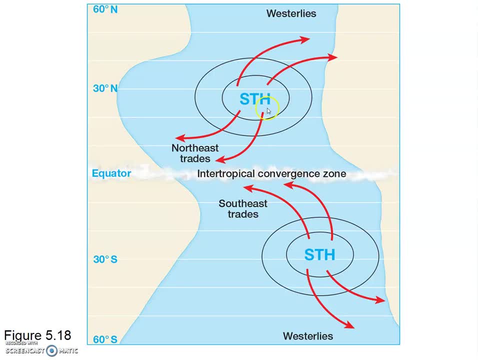 this mind where's when they are coming to a point 19 unique patterns. But if you look in the zone and the northeast trades are coming from the northeast into the intertropical convergence zone. Refer back to the six pressure diagrams I asked you. 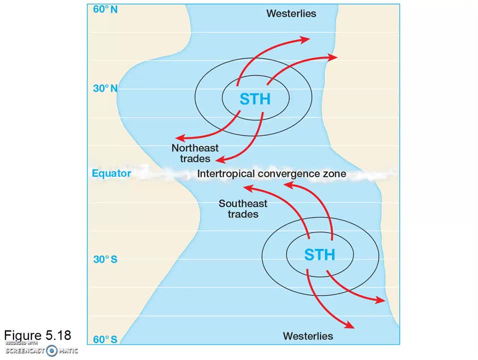 to draw on the previous video clip. You drew them right. Look at your diagram of surface winds: lower atmosphere winds in a high-pressure cell in the northern hemisphere. From a high-pressure cell in the northern hemisphere the surface winds would be clockwise and divergent. Now look again at this diagram. A high 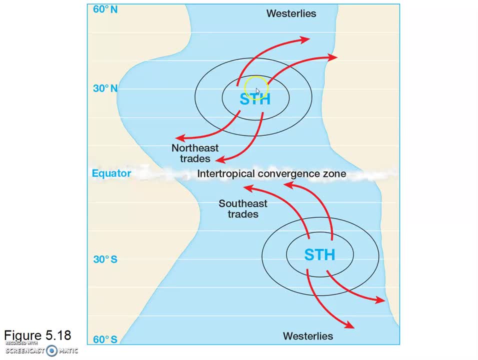 pressure cell, the surface winds are clockwise and divergent. Indeed, these here, coming from the subtropical high, diverging outward in a clockwise manner towards the intertropical convergence zone, are our northeast trade winds, And we see the mirror image in the 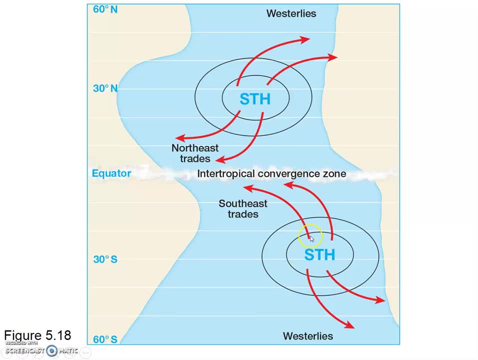 southern hemisphere, remembering that the the direction of the winds is going to be reversed, so it's counterclockwise here- but diverging outward towards the equatorial area of the intertropical convergence zone. Those are, the southeast trades. Lastly, look at the other wind that's created from the 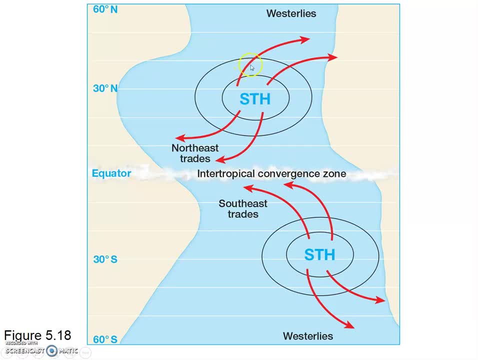 subtropical high, as the air is diverging outward in a clockwise direction. This is going to be the westerlies, the next wind that we deal with. So, really, if you can draw the diagram for a high-pressure cell in the lower 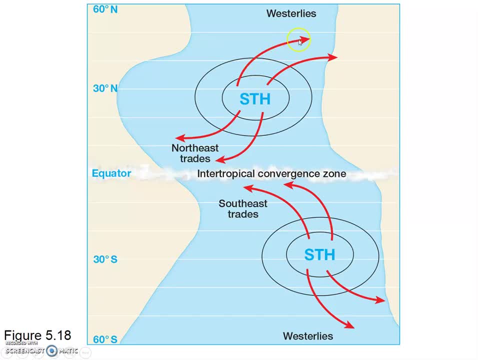 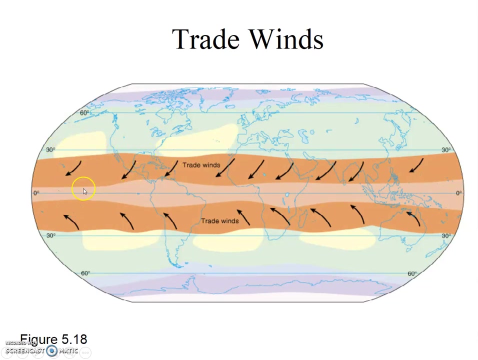 atmosphere, winds and a high-pressure cell showing the divergent clockwise flow. that's the crux of understanding much of the global wind and pressure system. You can see the trade winds in this diagram flowing from 30 degrees north, the subtropical high, to the intertropical. 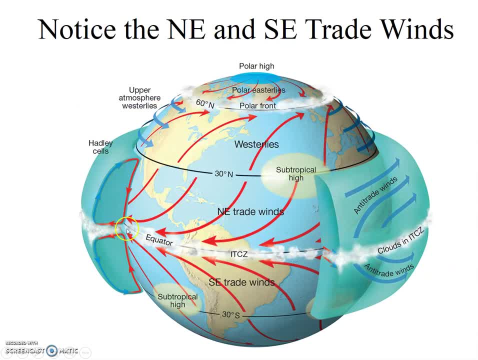 convergence zone near the equator And we can see them again in this diagram here, All these diagrams showing the same thing. The intertropical convergence zone is a low pressure, subtropical high is a high pressure and the winds are diverging out of that subtropical high and converging at the 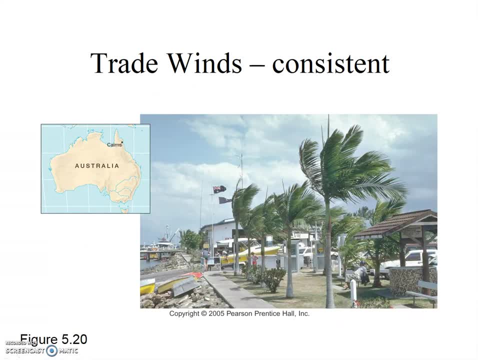 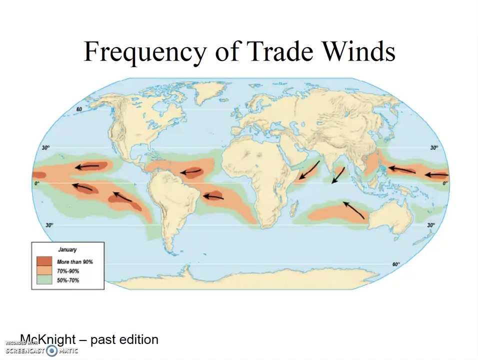 intertropical convergence zone. The trade winds get their name because they were used for shipping trade back when we relied on ships to move products around the world. The trade winds are very consistent so they were reliable to use for shipping. You can see in this diagram here that the frequency of the winds 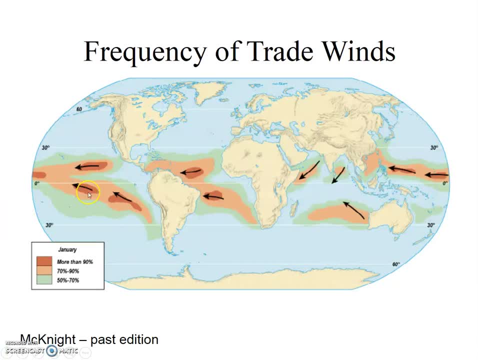 more than 90% of the time, the winds in in these darker red regions are flowing in the manner consistent with what we would predict from the trade winds you 70 to 90% is shown in orange here and 50 to 70% is shown in green. 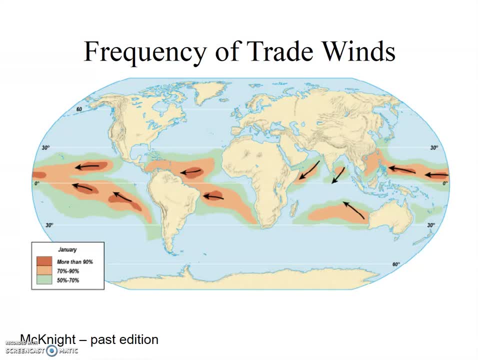 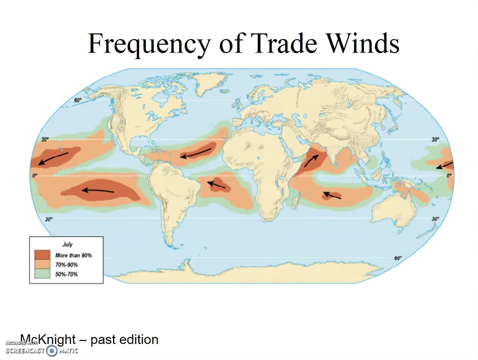 Again a very consistent wind, at least in January. Check out what happens in July. Most of the world remains consistent in terms of very consistent trade winds, but there's one place that it actually reverses, and we'll talk about that in. 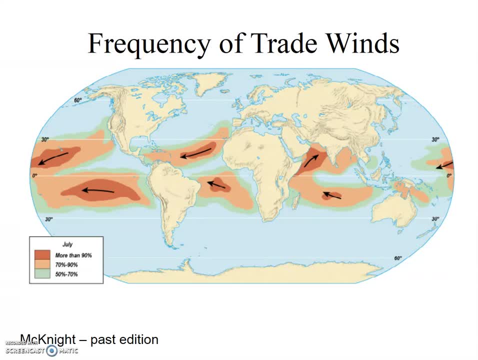 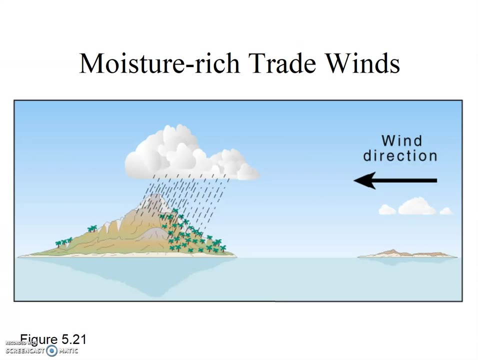 a little bit later, when we talk about monsoons, See if you can find the place where the wind actually reverses direction in July and think about why that might happen. Also, notably, the trade winds are warm winds that flow for thousands of miles over warm oceans. Thus they're full of moisture. However, they 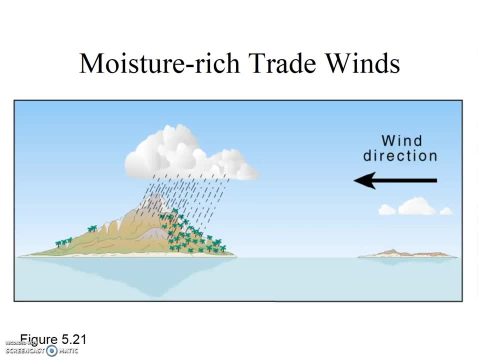 don't always result in rain. The trade winds are very consistent, so they're very consistent with what we would predict from the direction in July. Also, they're full of moisture, However, they don't always result in rain. In order for rain to occur, the air must be lifted by convection or some topographic barrier, etc. in order to cool enough for condensation to take place and for precipitation to fall. 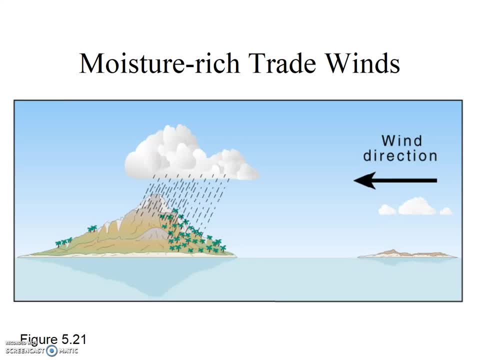 But if this warm, moist air is forced to lift, you can get really heavy rainfalls. If you've ever been on the big island Hawaii on the eastern part of the island, you know that it's a virtual rainforest on the eastern side of the island.